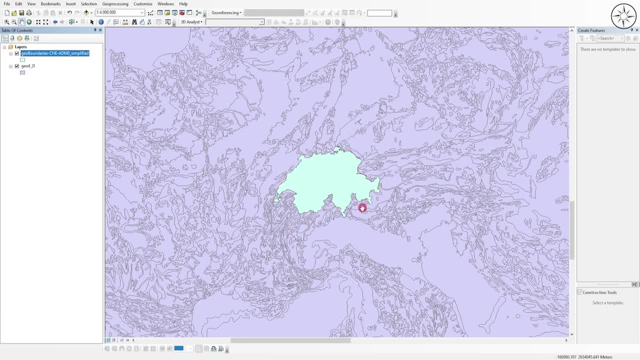 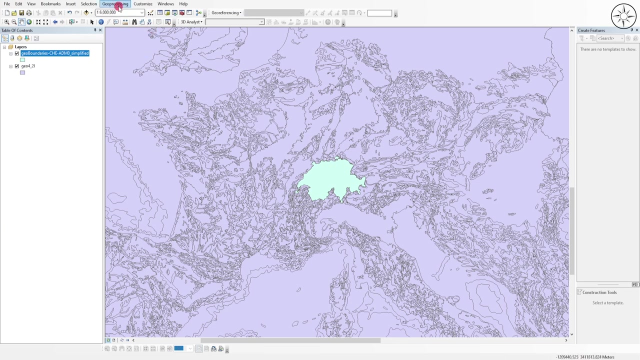 this is the shapefile boundary of switzerland. If you want to know how to download this file of any country, you can watch my video on how to do that. So I'm going to clip the geology of switzerland. in order to do this, Go to geoprocessing and then click on clip For the input feature. we 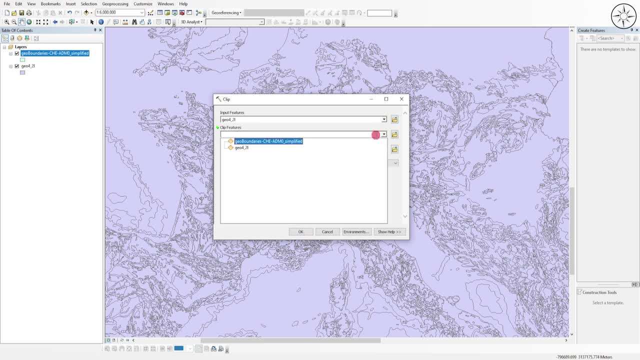 are going to input the geological map of switzerland. So I'm going to click on the geological map of the geology of europe And for the clip feature we are going to put the shapefile of switzerland. So here you can specify where you want to save your output. Click on name it, click on save. 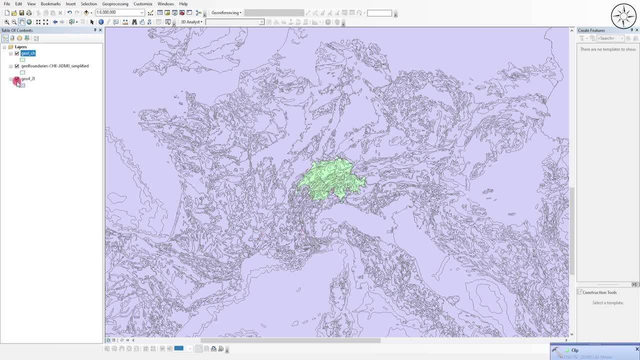 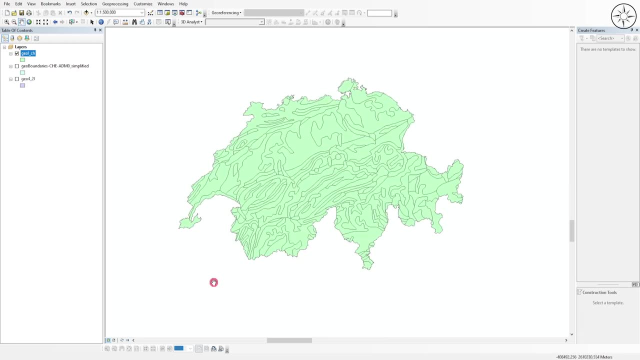 and then click on ok. At the end of this operation, you will get the shapefile containing the geology of switzerland. From here. I am going to use the layout view in order to make a geological map, So click on this small button next to data view. 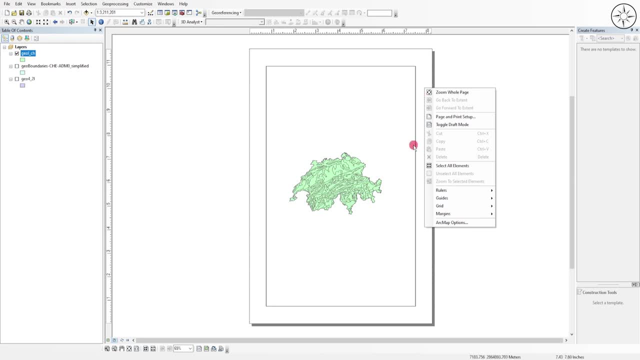 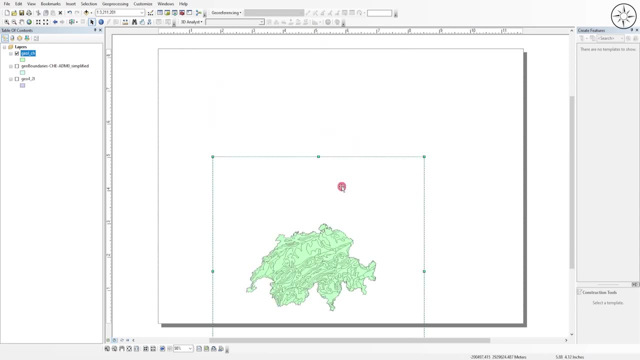 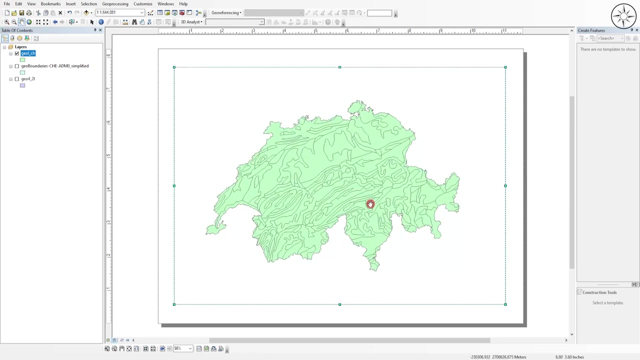 It's layout view. So here I'm going to change the print setup: Click on landscape and then ok. Then I will go ahead and resize my frame. Okay, I will zoom into my map. So the first thing that I'm going to do is to create the legend of this geological map. So I will open the attribute table. 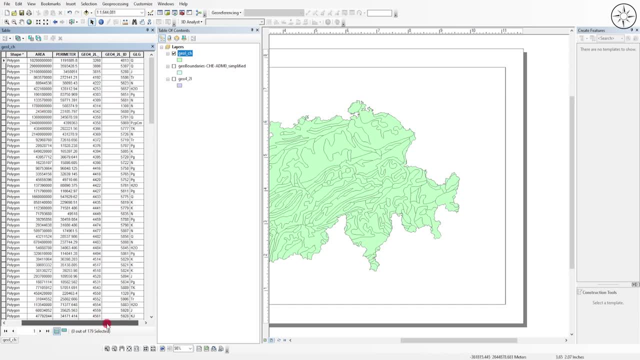 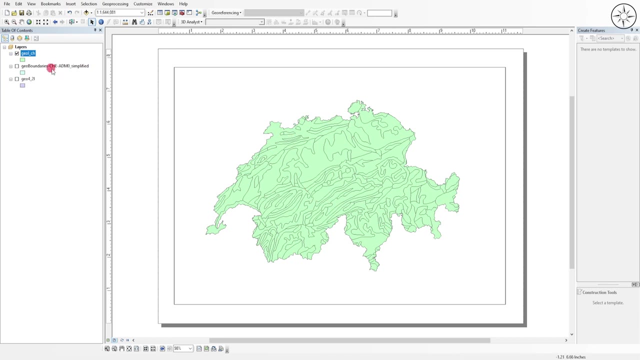 of this shapefile. As you can see, we got a bunch of columns, but the most important column for us is glg column, which contains the geological formations, So I will go ahead and create a new legend for this map. In order to do this, go to your shapefile layer, click on properties. 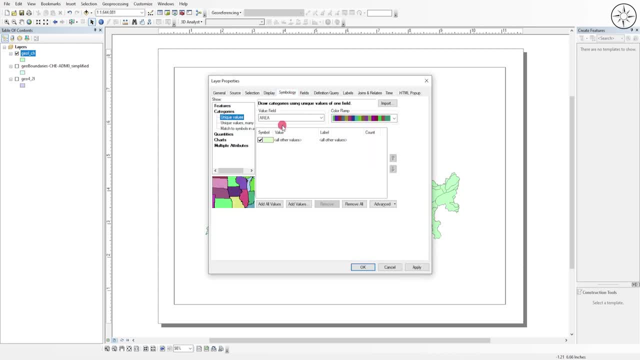 and then go to symbology and click on categories. Here, for the value field we are going to put the glg, which stands for the geological formations, I will click on add all values. As you can see those geological formations of our geological map utilizando google parameters will check if they. 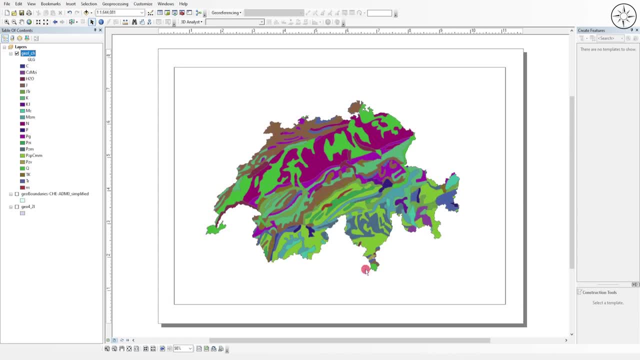 will check the other values too, Click on apply and then ok. So, as you can see, we got our technological map with the color of each geological formation. So I will start by adding this legend, I will go to insert and then we'll click on legend. So we'll go ahead. 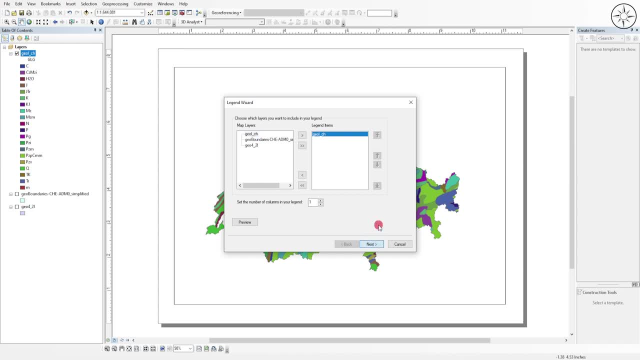 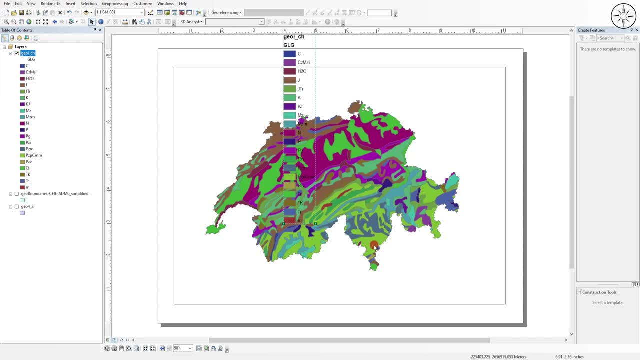 and put only the legend of our shape file. I will click on next. This is the title of my legend. Click next. i will then again click on next, next, then finish. so here we go. as you can see, i got my legend right here, so i will get rid of this title. i'll click on your legend. go to properties. go to: 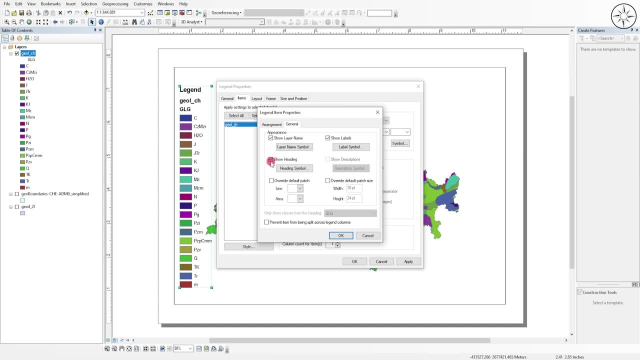 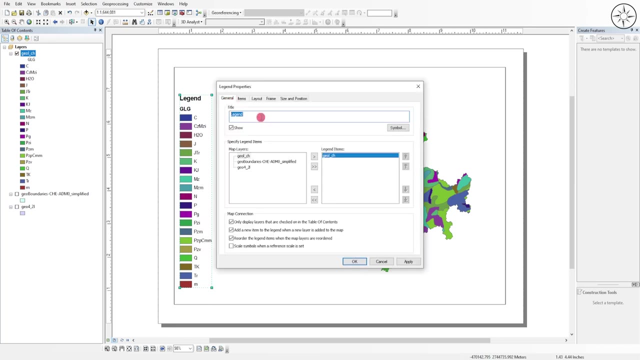 items. right click on your layer, go to properties and i will, and select show layer name. then i will click on okay, apply, and then okay, i think i will remove the title of my legend. go to general, delete the title, click on apply and i will even remove the second title. i will uncheck. 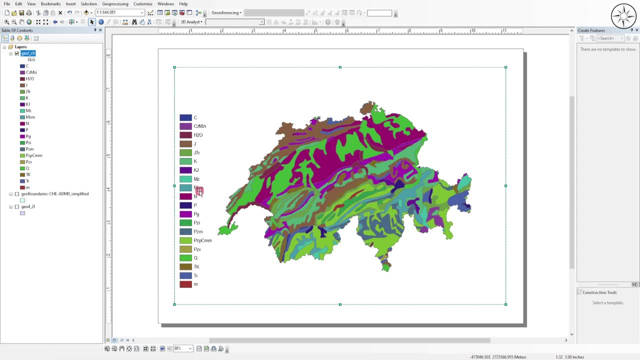 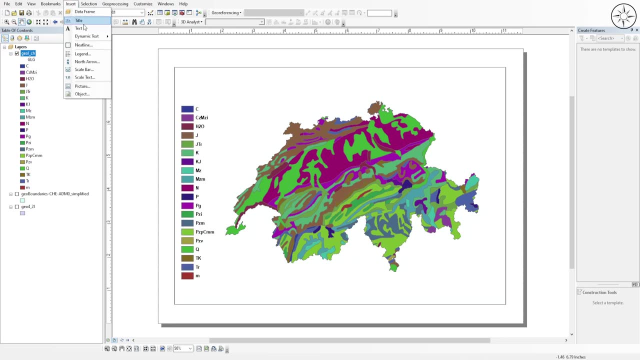 show hidden. click on apply and then okay. so this looks perfect for me. i will go ahead and insert, for example, the north arrow. click on north arrow. i'll go ahead and use this one. i will put it here. increase the size. i will go ahead and add a scale bar. 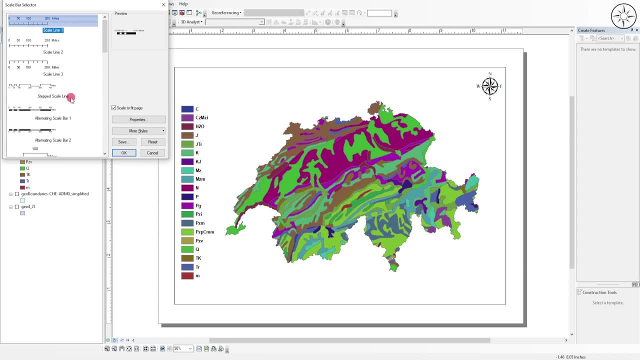 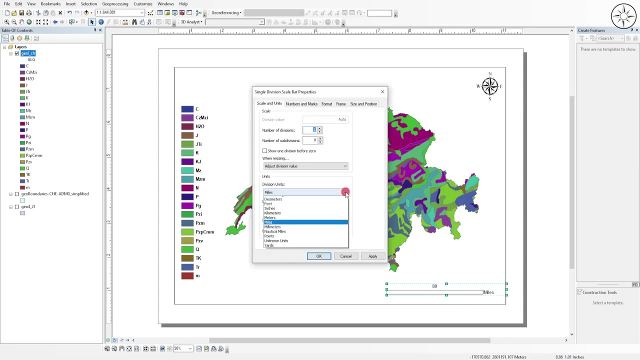 now go again to insert, click on scale bar. i will go ahead, for example, and use this simple one, click on ok, so we will modify this scale bar. right click on it. go to properties for the scaling unit. we'll go ahead and use kilometers for the level position we are going. 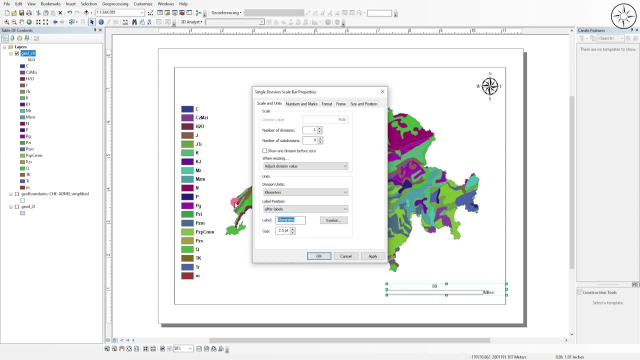 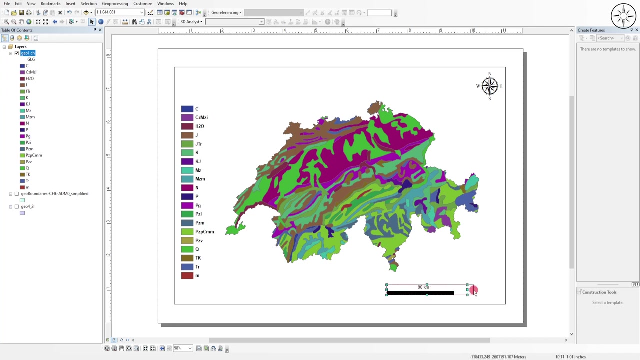 to put it after labels, and we'll put km for the numbers and marks. i will leave it to default for the format. we'll set the color to black, the fill color of our scale bar. i will click on apply and then ok, so you can play with the size of your scale bar until you find a suitable value. so 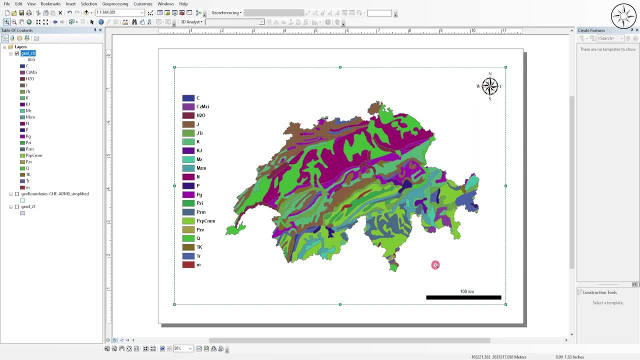 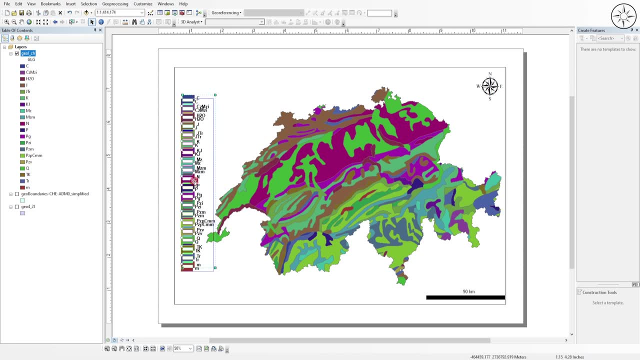 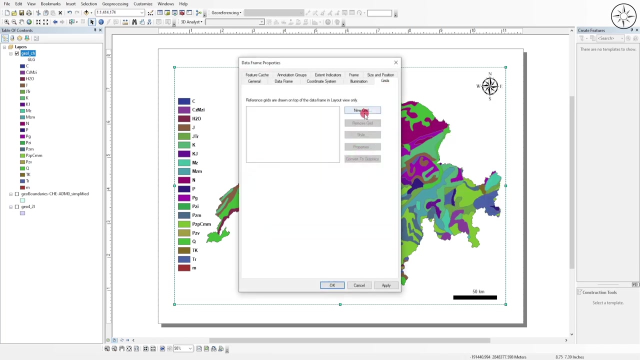 i will zoom in a little bit to fill the space inside of this frame. so here you go. i think that this zoom is perfect. i will resize this scale bar. i will go ahead and put coordinates on this frame. in order to do this, click inside of this frame, right click and go to properties, click on grids and we will.